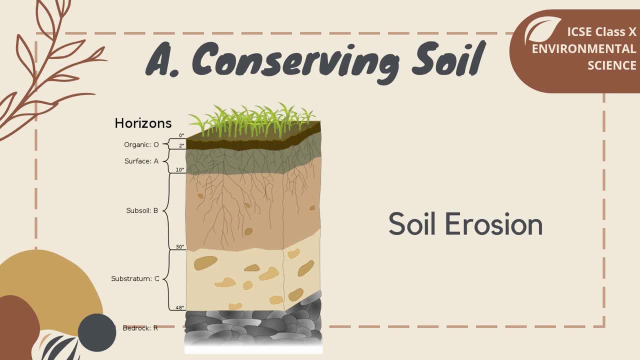 soil. Now, when we see the layers of soil, the topmost layer is the O layer or the organic layer, the layer which is really rich in organic matter, and then we have the surface A, or which is also called as the top soil, which is comprised of minerals plus organic matter, plus all the organisms. 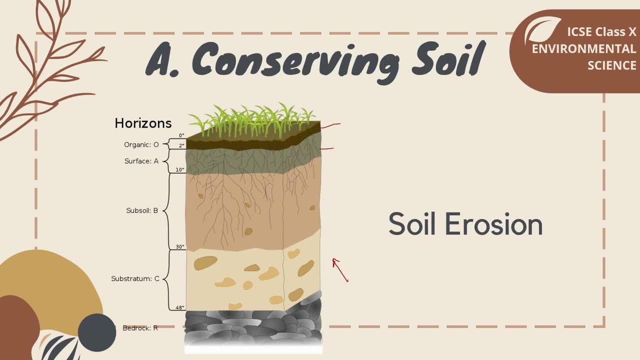 Now, when we talk about soil erosion, soil erosion is where the top fertile layer gets removed from a particular area. so when we talk about soil erosion, we are basically talking about the removal of both O and A layers. these layers, these really rich fertile layers, are getting removed. 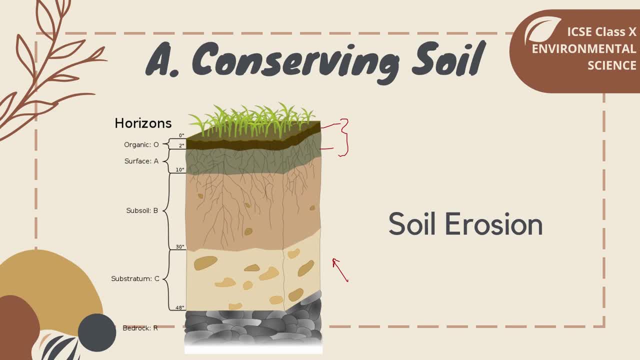 from a particular area due to several agents. it could be due to rain, wind, due to human activities, any of the above- but then the problem is that these are the fertile layers, these are the layers which are supporting plant growth, and they are getting removed, washed off from a 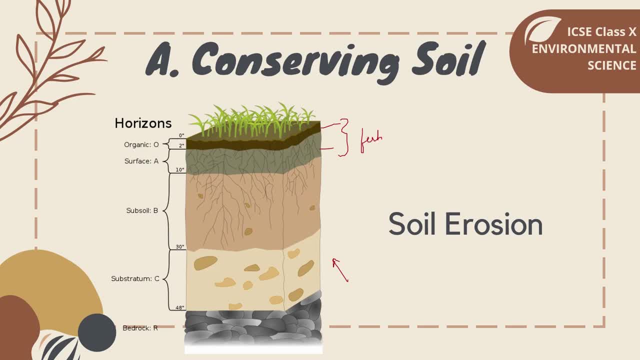 particular area. Soil erosion is one of the major concerns that are there with respect to conservation of soil. so when we say that we want to use it in a rational manner, we want to use the natural resources rationally or equitably, without degrading them. we want to have a sustainable use. 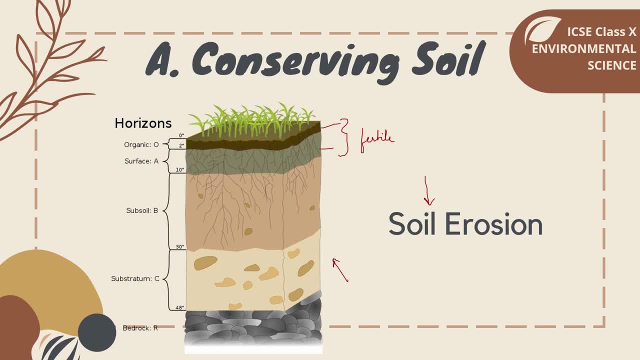 of soil. the major hindrance that comes over there is soil erosion. So we'll talk about what are the different management factors that are involved in soil erosion, and then we'll talk about the management techniques, or how can we manage soil erosion in a better manner. how can we? what are the 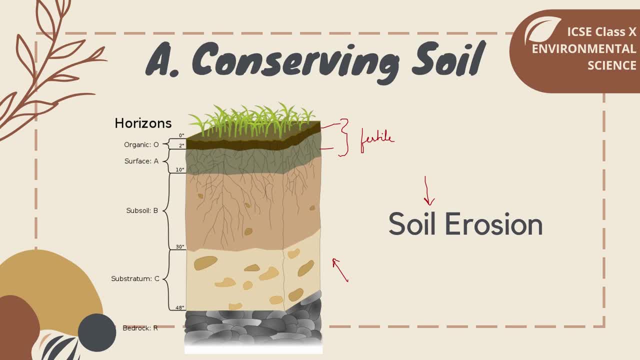 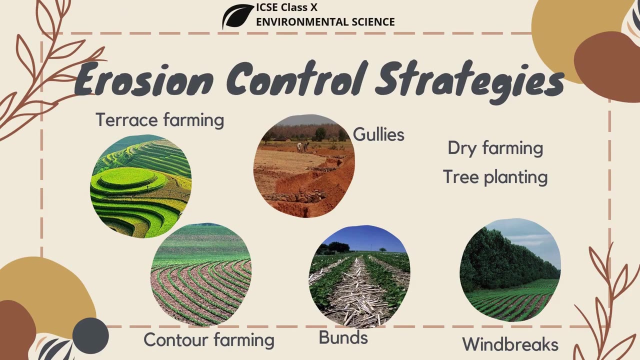 different control strategies that are there. So what is the problem with soil erosion? see that we have already seen the causes. we know that. you know. deforestation or over grazing or any other activity that is related to urbanization or industrialization or population growth, for example, over mining- can be a cause of soil erosion. Improper usage of land is a cause of soil erosion, but 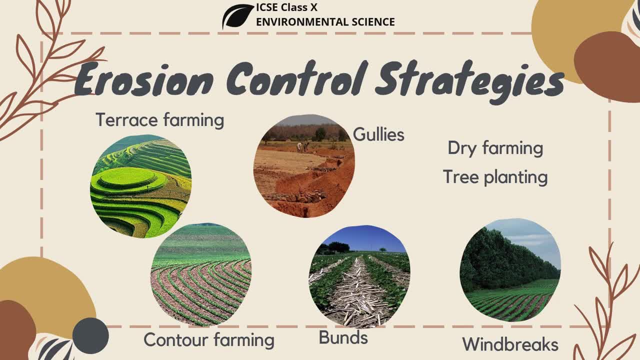 what exactly is the effect? why are we worrying about it so much? so we already saw that the top layer is being removed, so there is loss of fertility. that happens in a particular region. secondly, it affects the water holding capacity. There are no plants which can grow in a particular 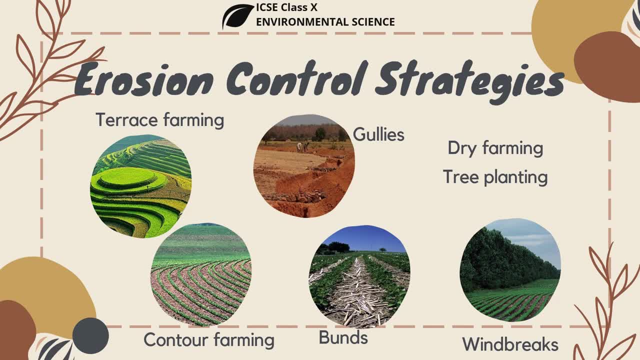 region, automatically water holding capacity of that soil goes down and you also have silting of water bodies because all of the soil in a particular region is reduced to a certain level. Remove and it goes and gets deposited in the water body and it causes silting of water bodies. 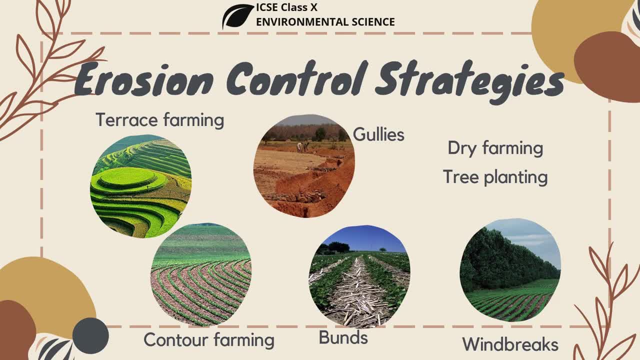 So these are some of the effects that can happen due to soil erosion. there are much more bigger effects, like desertification, which we will deal with in a different video. but the reason we need to control soil erosion is mainly because it causes fertility loss in a particular region. So what are the different control strategies? the first one is: 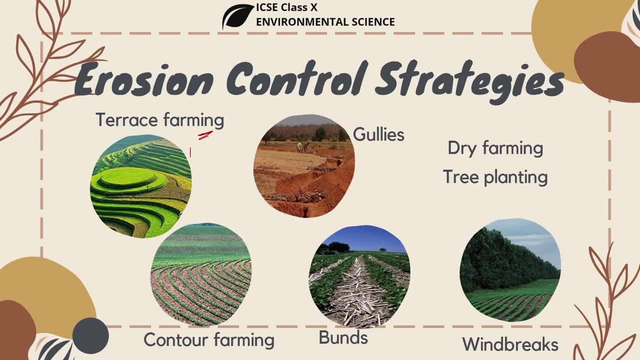 terrace farming. Terrace farming is something that we see mainly in the hilly regions and it can be followed every anywhere, but then hilly regions is where we usually see wherein the fields or the entire land has been cut at right angle, so you can see some sort of- you know, steps that have been. 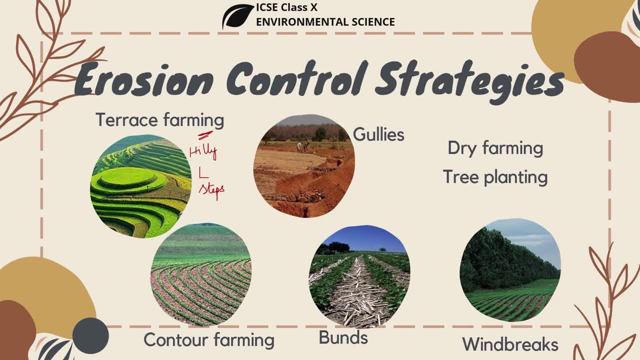 formed into the land itself, and these steps, or these terraces, which we call, are the areas where agriculture is being carried out. so the agriculture is carried out on the flat surface and this is really good because it reduces the runoff of the water. it reduces the water from getting, you know. 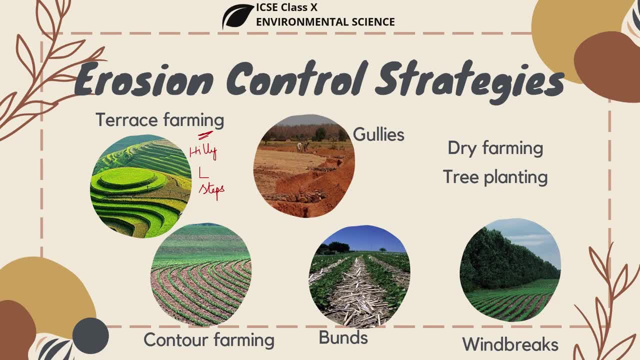 the soil erosion. The second one is contour farming. contour farming is similar to the terrace farming, it's just that here you don't cut at right angles. instead you are tilling the. you know the slope land along the lines of the elevation. so if the, if the land is having a 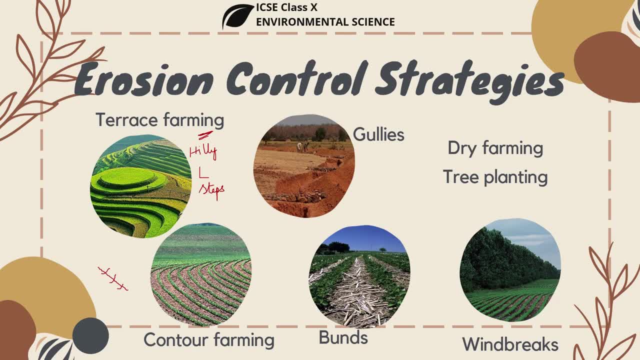 slope like this along the elevation of the land, if you're growing, if you're tilling the land and you know having farming over there, or if you're plowing the land in, that is according to the contour of the region. that's what we call as contour farming. Again, here, 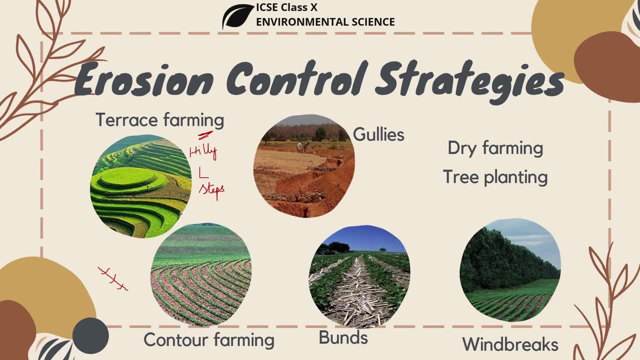 it's prevent soil erosion because it acts as a reservoir. these areas act as a reservoir to catch the rain water, to retain the same rain water, so it ensures that you know the water doesn't flow down taking the soil along with it. instead, it goes into the soil. The third one is dry farming- dry. 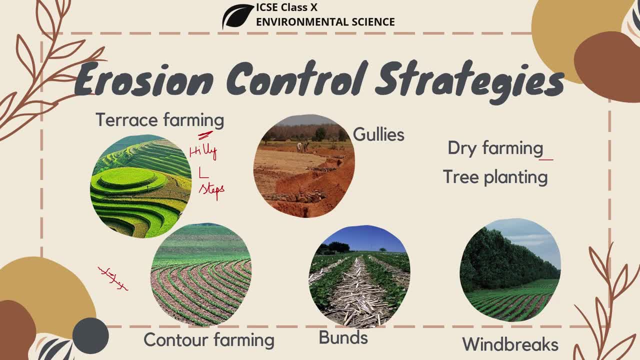 farming is mainly followed in the arid regions or semi-arid areas where the rainfall is not very good, where they have, you know, rainfall in the rainy season, but then the rest of the year is really dry. In these reason regions you don't have irrigation, you do not use irrigation, you do the farming with. 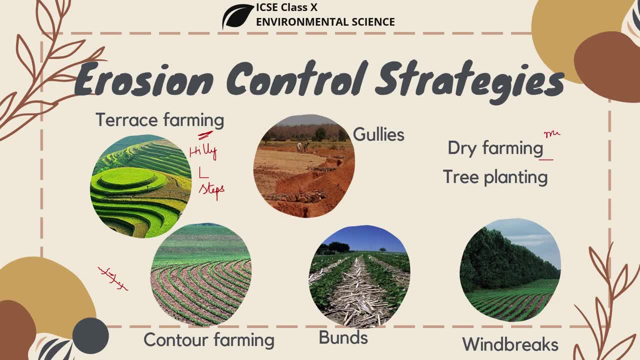 the help of moisture that is retained within the soil. so whatever moisture is there in the soil is what you are using. that is called. if that's the technique that you're employing, then that we call as the dry farm. Dry farming mainly ensures that you use drought resistant crops, or you are you. 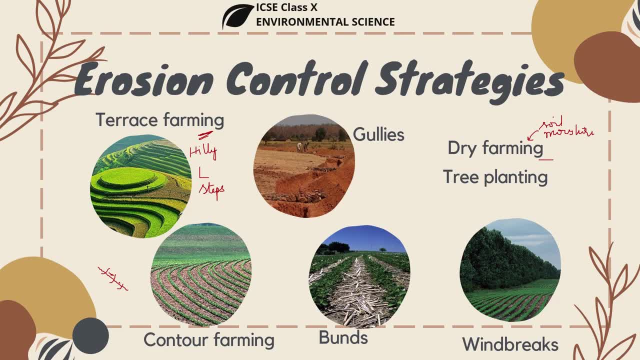 know, having some sort of mechanisms in place, like you have, applying a fine surface of mulch or the residue such that the water is retained in the soil, you are protecting that soil moisture from evaporation. that's what you're trying to do. that's what we call as dry farming. 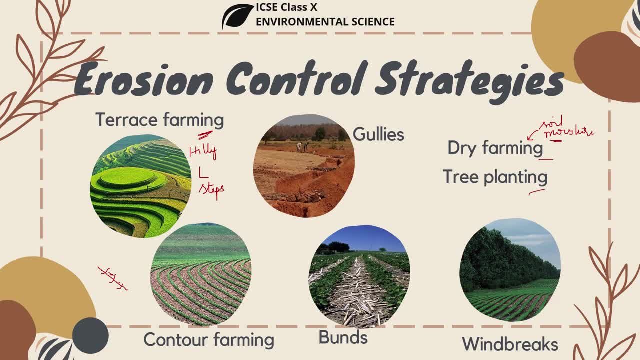 Tree planting is definitely is a method for controlling erosion, because the roots of the trees will hold the water in place, so transplanting the tree seedlings itself. it's usually done in areas where the forest was harvested or it was damaged due to some fire or disease. in such areas, 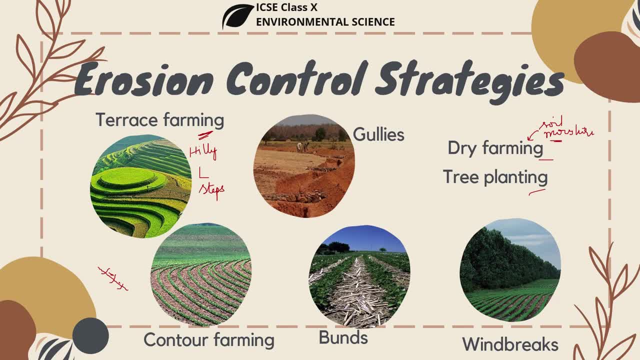 we go for tree planting, ensuring that the trees are going to provide water from the dry soil, which is a great source for agaric plants, prevent the erosion, or you know, the organic matter in the soil is increased and that not only prevents or reduces erosion, it also reduces pollution and provides a natural habitat. 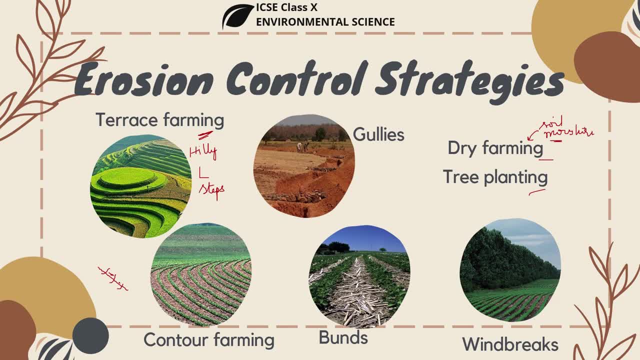 for the biodiversity. The next one we have is the formation or use of bunds. Now, bunds are basically barriers, so these barriers could be in the agricultural land. you could be making it of stone, it could be made of soil or, like what's shown over here, it could be made up of the crop. 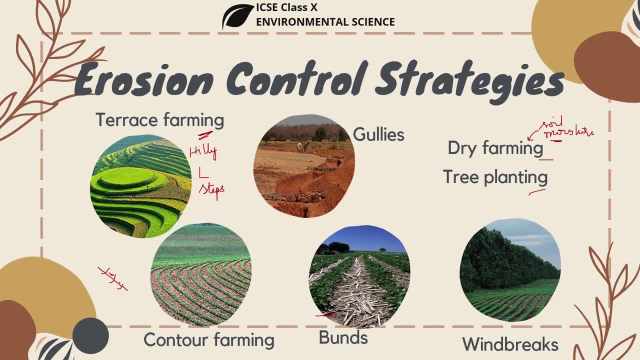 residue itself. So these bunds are basically acting like a barrier to control the rainwater, allows the water to get infiltrated into the soil and thus prevents erosion. Something very similar to bunds are the gullies. Gullies are trenches or ditches which are, or channels which are dug into. 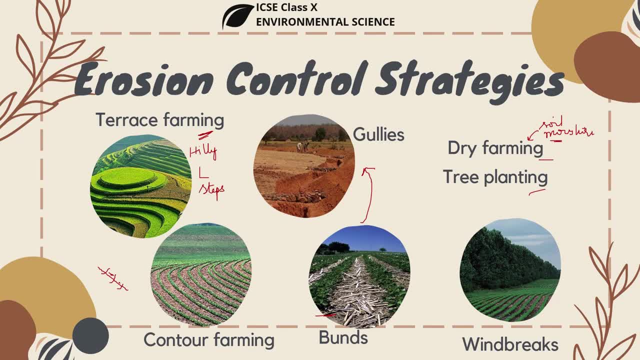 the soil. So these channels are again cut into the soil so that rainwater does not, you know, go keep flowing. it gets collected in that channel and, you know, after a heavy rain or after a downpour that channel will now get filled with rainwater and that can later be used for irrigation or for 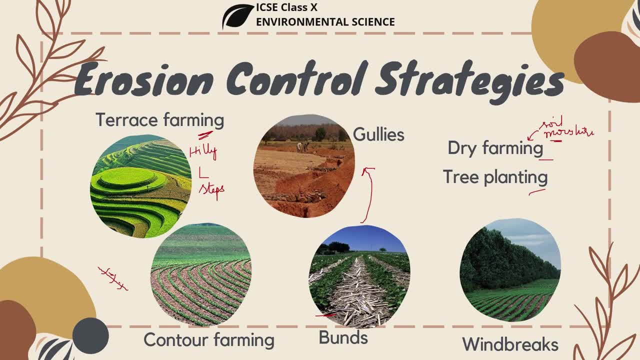 any other kind of purpose. So gullies and bunds are basically methods where you are trying to channelize or, you know, take the rainwater and use it for other purposes. We can even have windbreaks, or windbreaks are also called. 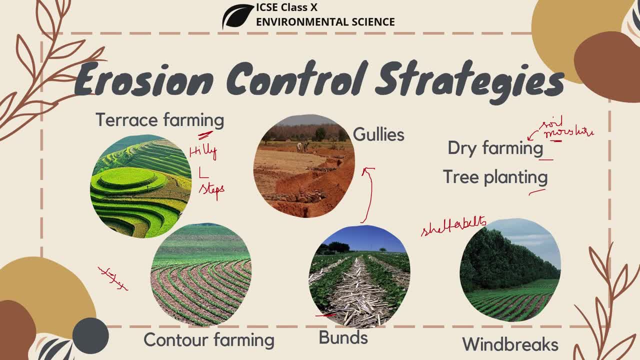 as shelter belts. Shelter belts, like the names you know suggests, or windbreak, like the name suggests, is basically a row or number of rows of trees or shrubs which are planted at right angle to the prevailing wind. So if the wind is coming in over here, say this is the direction of the wind. 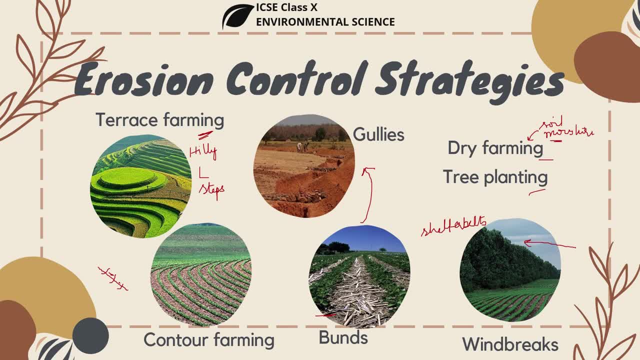 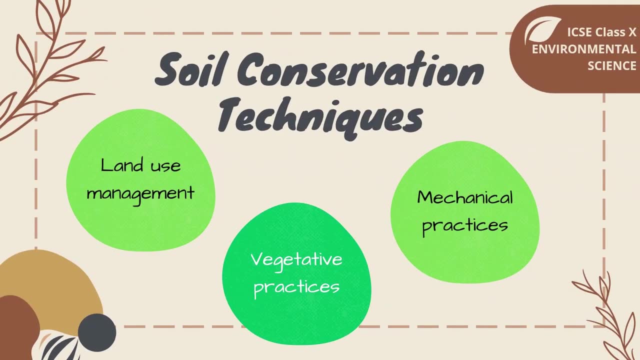 that wind is now going to get broken. the flow of wind is going to get broken because of these trees, which prevents the soil erosion in the nearby farms or in the nearby fields. So this is very important for reducing the velocity of the winds. Now, when we see the soil conservation techniques, 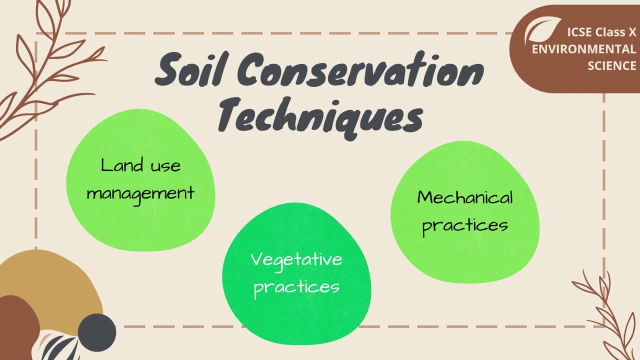 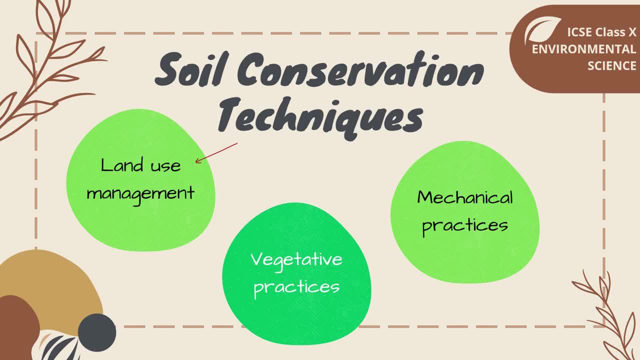 protecting the soil from the impact of the rain or from the impact of the wind, you are ensuring that more water goes inside the soil and it doesn't cause soil erosion. that's what you're trying to do: to decrease soil erosion, to decrease the volume and velocity of overland flow of water. that's what you're. 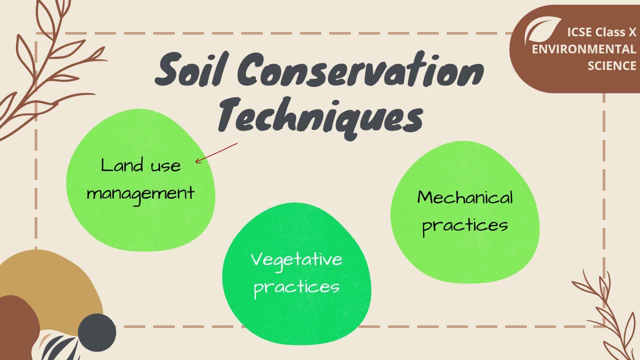 trying to do in these techniques. so the first method, or the first, you know way in which you can conserve soil is by land use management. now, land use management is you basically using a land within its capabilities. so you could have see there are different types of land use. you could have cropland, 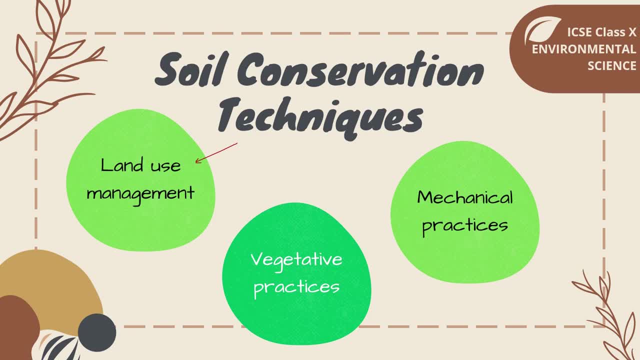 pastureland, woodland, wildlife land, recreational land, different types. you can use the land for different purposes. but what does land use management mean? it means you manage and you use the land. you develop the land resources in such a way, in the rural and in the urban areas, in such a way that you are even when you 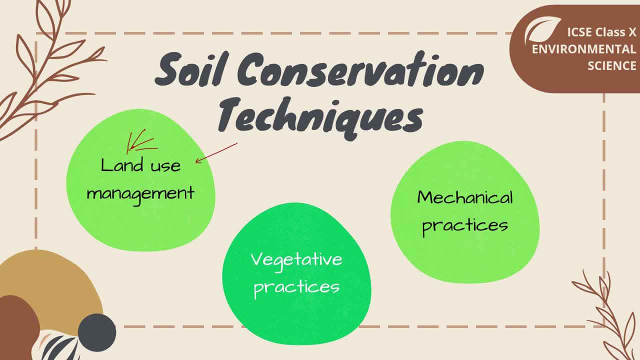 are, you know, converting from one form to another form, you are not posing a risk to the particular land. so, using the land within its capabilities. see, there could be one land which is a cropland. when you're converting it into a land where an urban land, you ensure that the soil erosion. 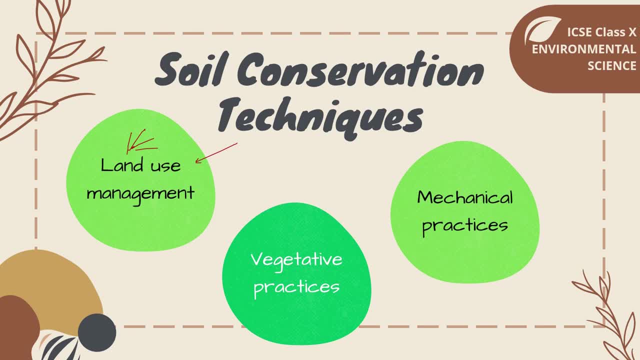 does not happen, you ensure that there are techniques in place which retain the rain water. so that is what we call as land use management. whenever land is being converted from one use to the other, ensuring that it is susceptible to erosion at that time. So you are ensuring that the land use management is being done properly. 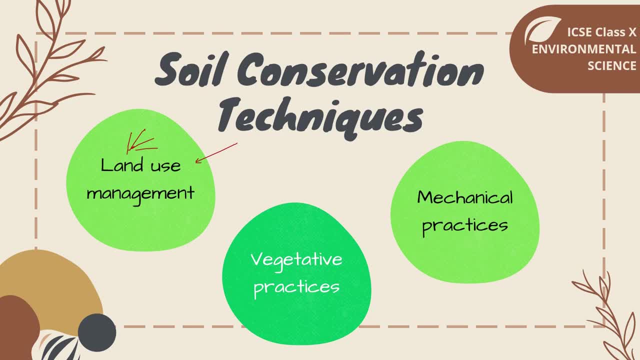 You are developing the land resources, you are converting from one form to the other without harming or without hampering the land. That is what we call as land use management. The second one is using vegetative or biological practices. Now, vegetative practices are basically the cropping practices. 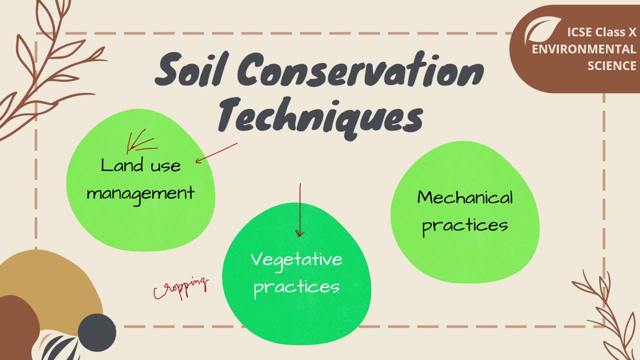 So you use different types of cropping techniques, For example, crop rotation or alternate cropping, or, like we saw in the previous slide, using windbreaks or strip cropping. So you use different types of vegetative practices to ensure that the soil is getting. 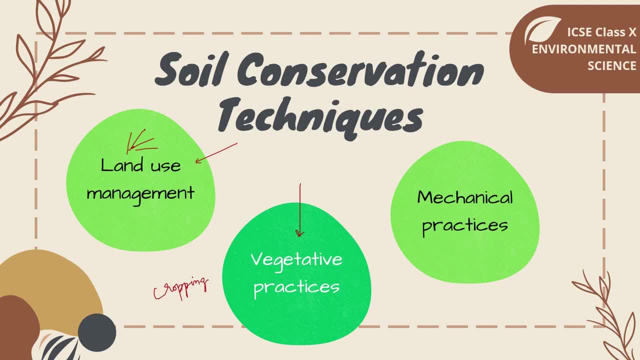 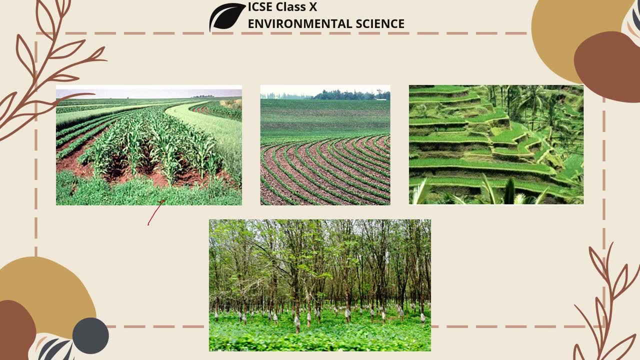 conserved. And the third one are the mechanical practices, which are basically engineering measures. So you can see over here the first one: what we have is a strip cropping, where you are using alternate strips of row crops and inter-tilled crops at right angles. 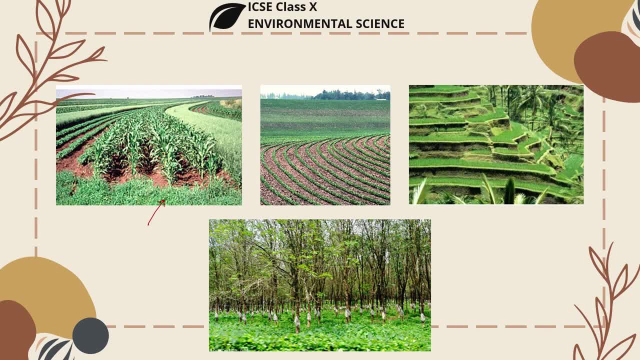 Basically, you are using different types of crops, you are using different rows of crops, ensures that the soil. Soil is not getting eroded very easily. it is also good for the fertility of the soil, Or even contour farming is a type of method, is a type of cropping practice, which is a 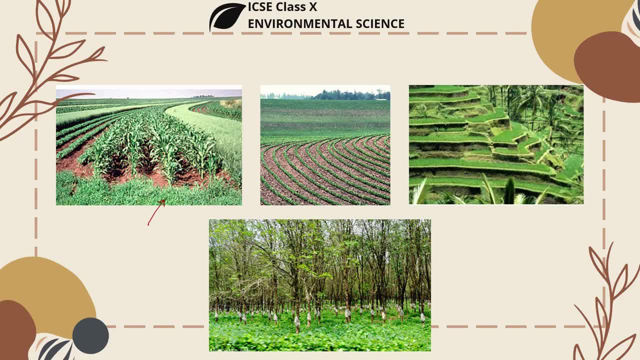 vegetative measure or terrace farming, like shown over here, or using the cover crops. All these are examples of the vegetative practices. Mechanical practices are basically engineering measures, like we saw earlier, using bunds or digging gullies or any other, or even terrace farming can be considered as an engineering measure. 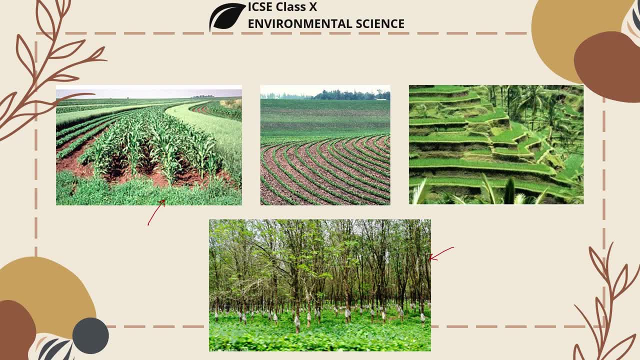 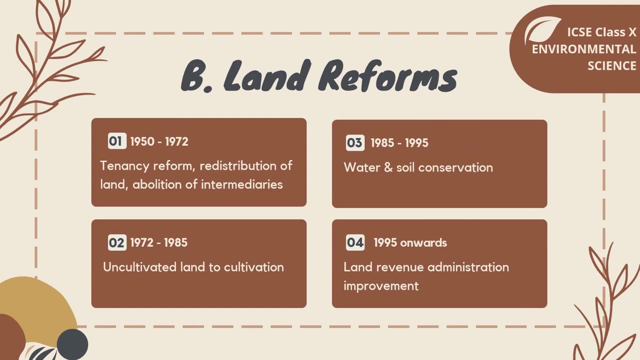 So these are examples of mechanical practices. So mechanical vegetative practices and land use management are the different soil conservation techniques. Now the next part we have in New York syllabus is the land reforms. See, land reforms are basically the different measures, or you know, reforms that have been 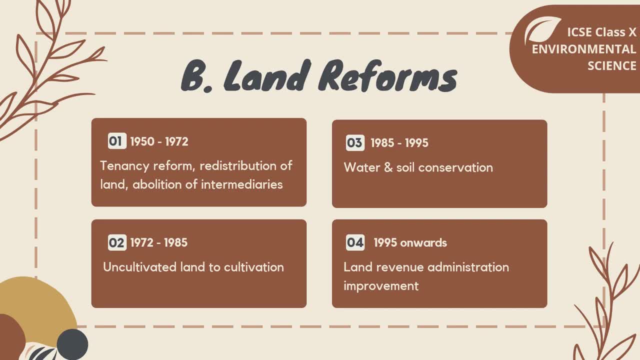 taken in India, to which are, you know, discussing the various changes that are happening, that have happened in India, In India with relation to land. that is what you call as land reform. So basically, this talks about the redistribution of land from the rich to the poor or anybody. 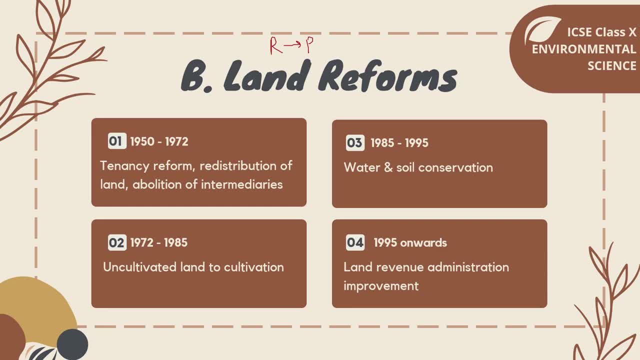 who is not having land. You are redistributing the land from the rich to the poor with the aim of increasing the productivity. That is the main aim: ensuring that the productivity of the land increases and also ensuring that poverty decreases. Both are. both of these are the aims that are in place, for you know, implementing any. 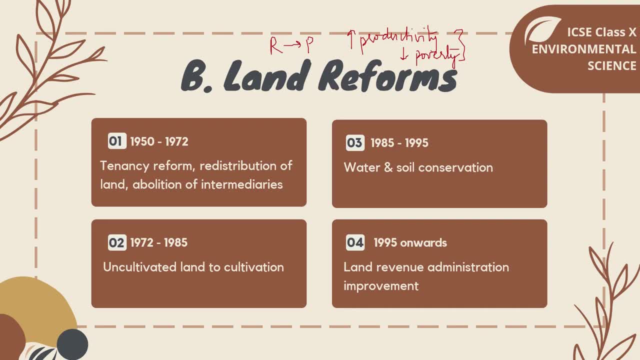 kind of land reform. So in India there have been multiple phases of land reforms and in India it is very, very important because we are an agrarian economy. We have a lot of land which is used for agriculture. Not only that, we have a large quantity of rural population which is below the poverty. 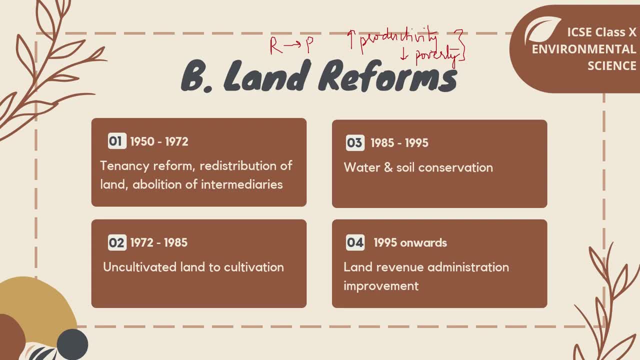 line. We have unequal distribution of land. There are rich have a lot of land and there is a huge section of poor people who do not have any land at all. So in India it has always been a top priority, at the time of independence and even in the 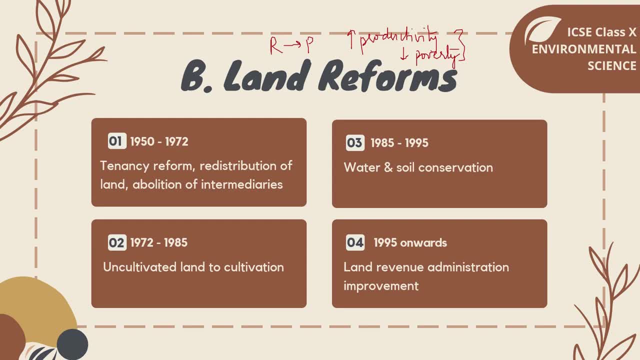 later decades to ensure that there are land reforms. So in India there have been four phases. I have showed it over here. The first phase, which is the longest phase, was from 1950 to 1972, which was mainly focusing on the abolition of intermediaries like the zamindars or the rent collectors to abolish. 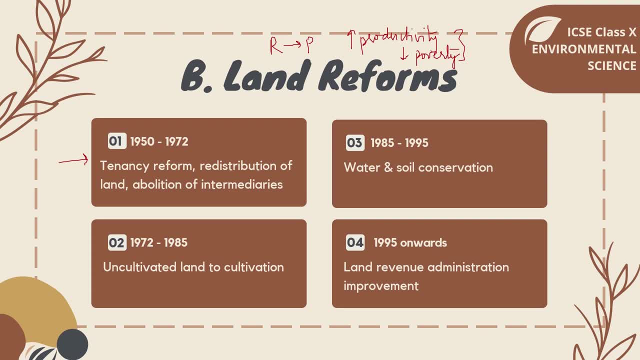 them so that the middlemen do not make money out of it. Second one was to reform the tenancy laws, that is, you know, to ensure or to give permanent creditable rights to people who are actually working on the field and redistributing the land using land ceilings. 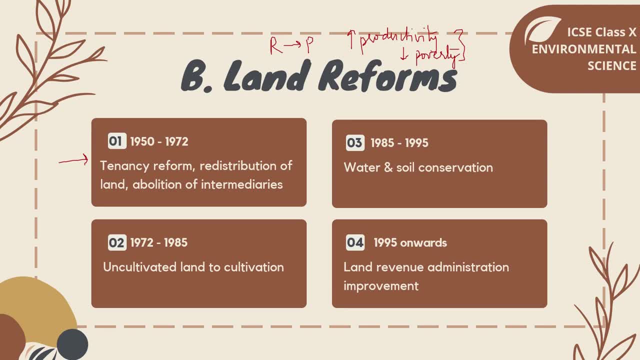 So these were the major aims that were taken into consideration during the first 2022 years. The next one was from 1972 to 1985, where the focus was on bringing the uncultivated land into cultivation, because the number of people was increasing and the demands were increasing. 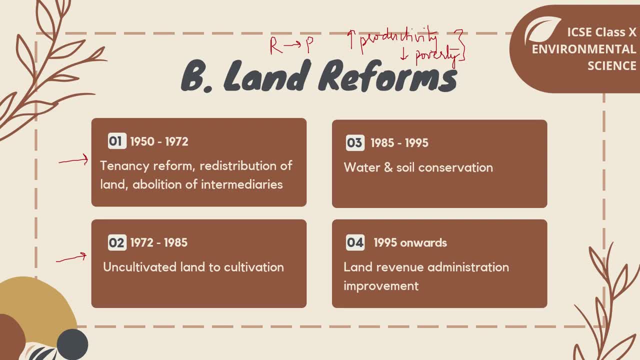 There was a lot of uncultivated land. How could we convert that into good fertile land Was the next phase. you know, focusing on. The third phase was from 1985 to 1995, wherein the focus was on conservation of soil and water. 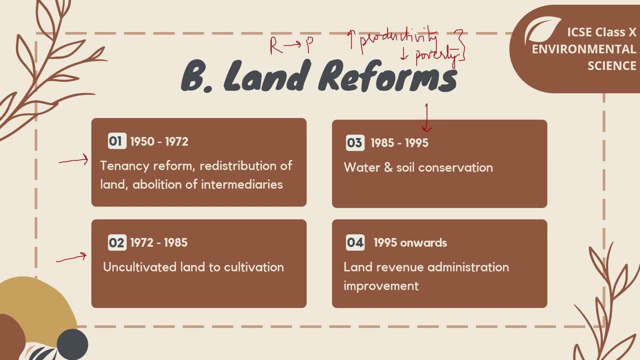 So, development of waste land, development of desert area, How do we ensure more of irrigation measures? This is what was taken care of in the third phase. The fourth phase, which is from 1995 onwards, it has been, you know, to improve the land revenue. 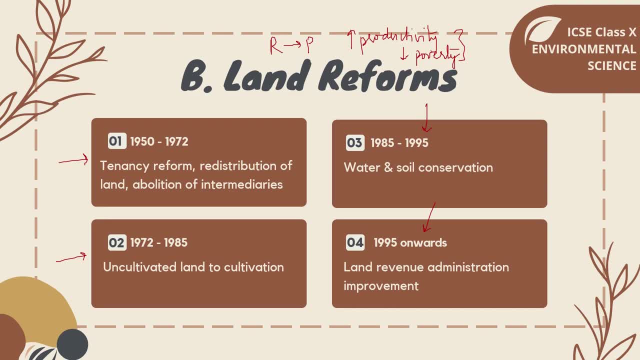 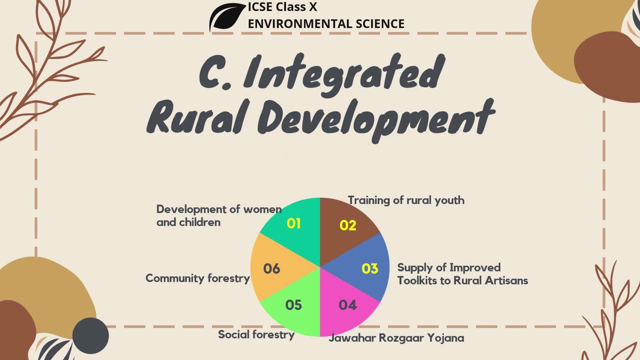 administration to continue the land legislation, especially the land records, Ensuring that land records are maintained properly. This is what we have been focusing on from 1995 onwards. So these are the different land reforms in place in India. So I guess this is the first phase. 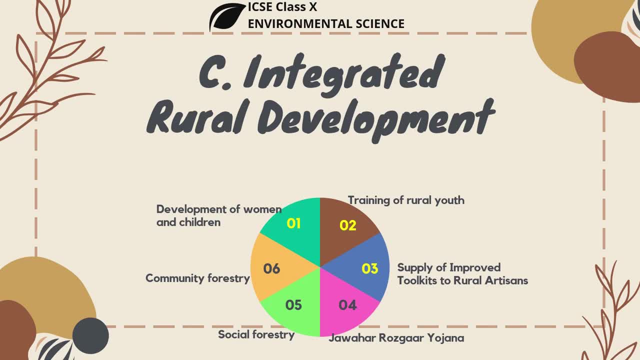 In India we started a program or we implemented a program called as the Integrated Rural Development Program. This was launched in the year 1978 and it kept on going till 1999.. After that we have rebranded it. So we do have that program now, but then it is rebranded into different schemes. 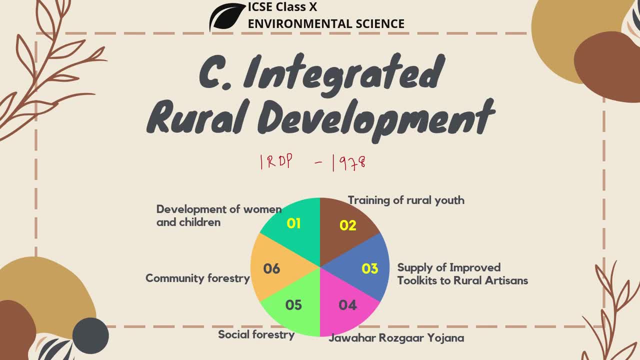 So this IRDP or Integrated Rural Development Program is basically a self-employment program. The main objective of it is to ensure self-employment amongst the rural population, amongst the rural youth, to raise their income, to raise their income generation capacity, to enhance their living standards, to provide subsidies or loans or some kind of credits to the target population. 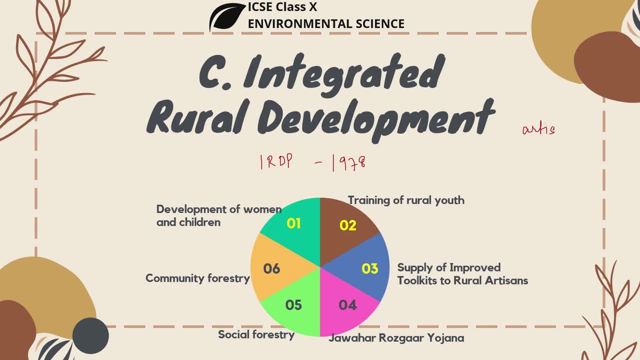 So the target population over here are the artisans who know some products. So the top percent who work in particular craft work are the people who are, you know, the labourers who are working in the rural region, or even the farmers, The farmers who are on the margins. even for them these schemes are intended. 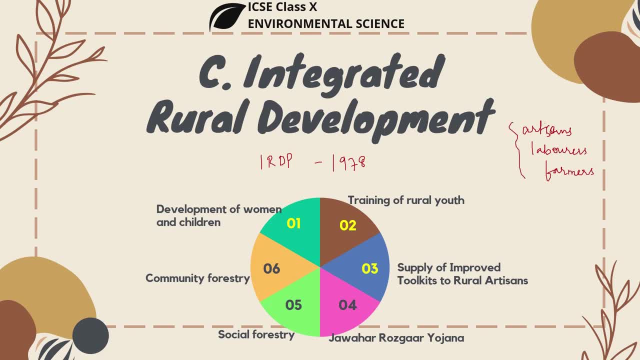 So the target population needs to come up in life. their living standards have to be improved, the income generation capacity has to be improved. These are the main objectives of the Integrated Rural Development Program. So under this we have defined that allness and知道ness. 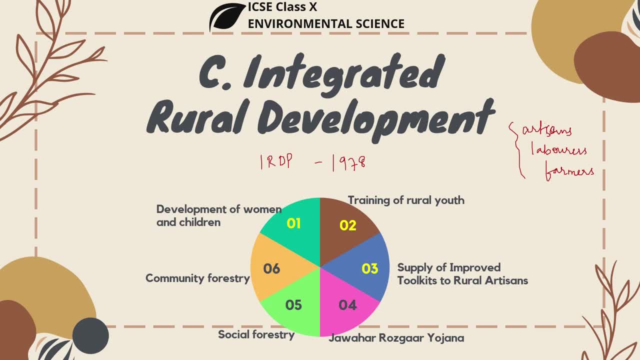 schemes that have been taken. I have just put up a few over here. there are many more. some of them include the training of the rural youth so that they are, you know, capable of self-employment, or the development of women and children in the rural areas, ensuring that there are sanitation programs. Jawahar Rozgar Yojana. 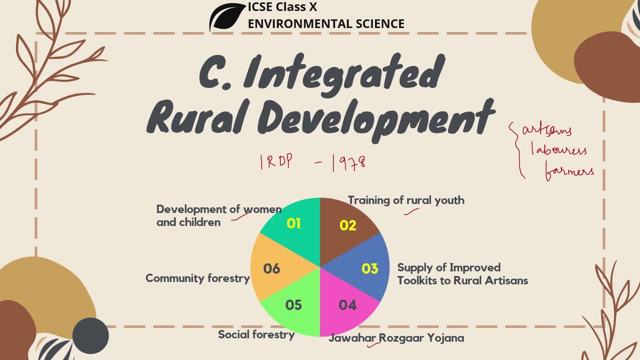 you might have heard of these. this is also for self-employment or scheme for the rural artisans to ensure that they are being provided with the improved toolkits. these are some of the schemes, but in your syllabus they have mainly focused on the social forestry and community forestry which we will talk. 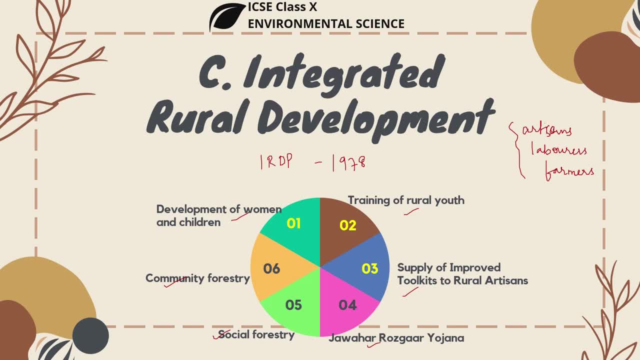 about in detail. so social forestry is where we use the unused land, the fallow land, the barren land which is not having any cultivation. we use that for growing fast growing trees. we want to grow trees that you know come up really quickly so that that those trees so on the fallow land you start growing trees which grow. 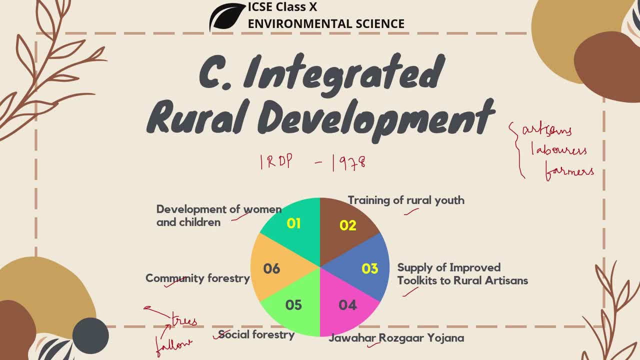 quickly, and those trees are then either used for fodder or they are used for fuel by the local community. this is what we call a social forestry. so you harvest those trees for the fuel wood so that the deeper forests which are present are safeguarded from exploitation, that is. 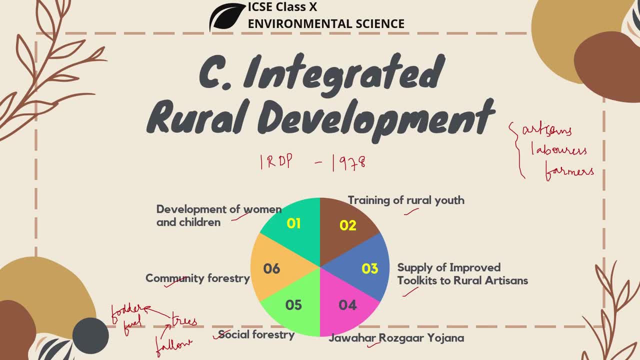 what we call a social forestry. what type of social forestry? so there are many types, but one type of social forestry is community forestry. community forestry is where, in the local people partake, or you know, to safeguard a particular forest. it may be a forest that they have planted, or it may be the forest. 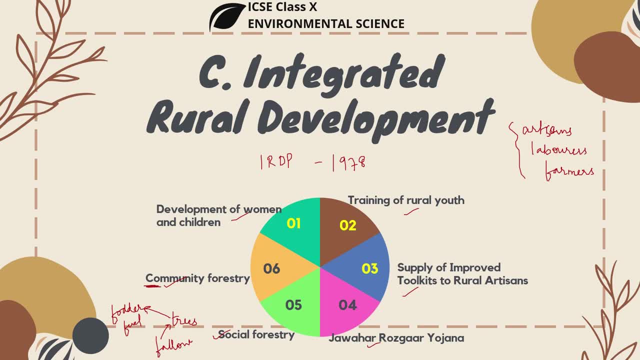 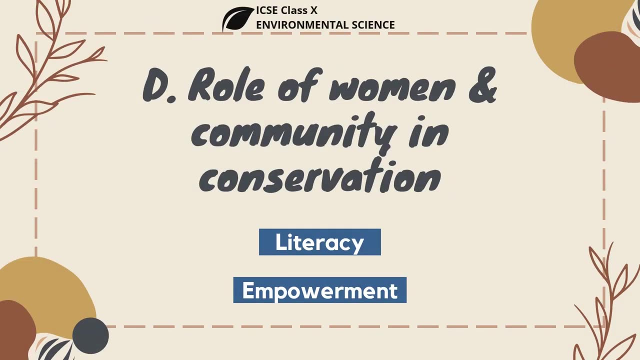 in general. but the local community participation is there to safeguard the forest, to improve the forest. that is what we call as the community forestry. so these are two schemes specifically mentioned under the integrated rural development program. in your syllabus is to know the role of women and community in conservation. so 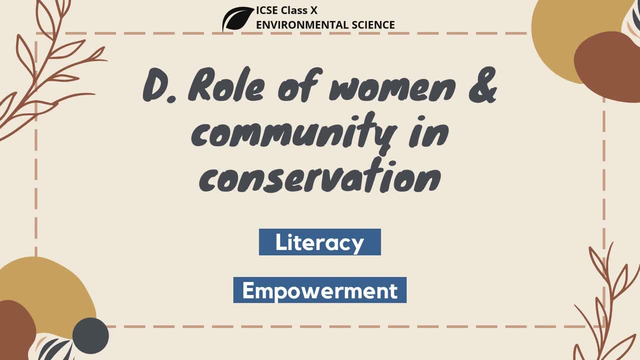 in general, the role of women is very, very important in bringing up a community or in conservation of the natural resources. the reason is because women are the ones who are directly playing, or you know, managing the natural resources at the grassroot level, because they play a very critical role, they are involved in. 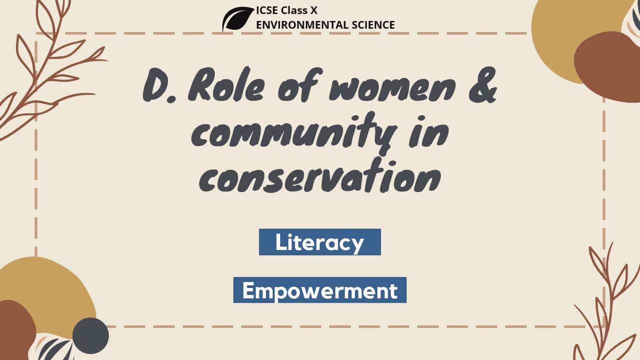 usage of water. they are based on some cases they are the ones who bring the fuel would. in some, in many communities, women are the ones who are preparing the food, who are collecting the food. so the role of women is very, very important in conservation of natural resources. if we ensure literacy, that is, if we make them. 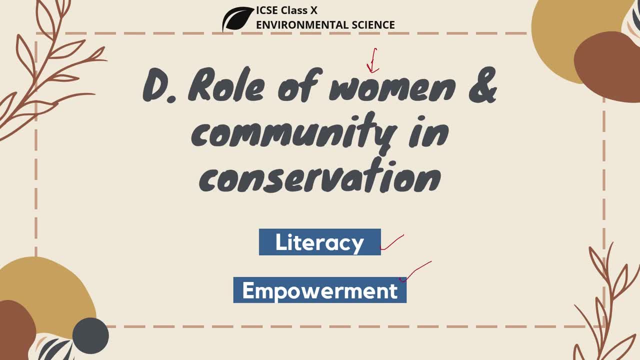 literate if we make them educated and we empower the women in any community it there have been reports which show that this leads to increased food production. the reason: because they adopt: once they are literate and they are, once they are educated and they are empowered, they adopt a scientific approach to. 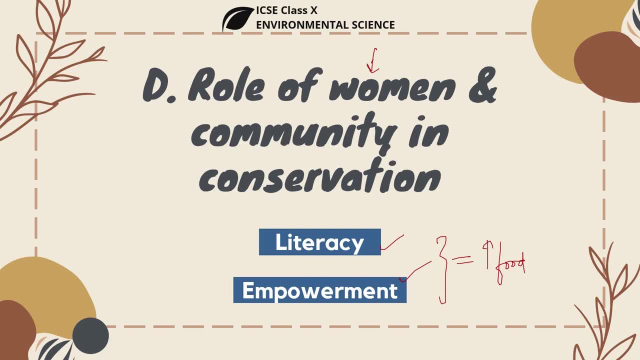 understanding things and that has helped, or that has shown, to increase food production in several countries, so even in India. we need to ensure that women are being empowered, you know they are being given an active role to conserve the natural resources or, in this case, conserving the soil, conserving the land, because women do. 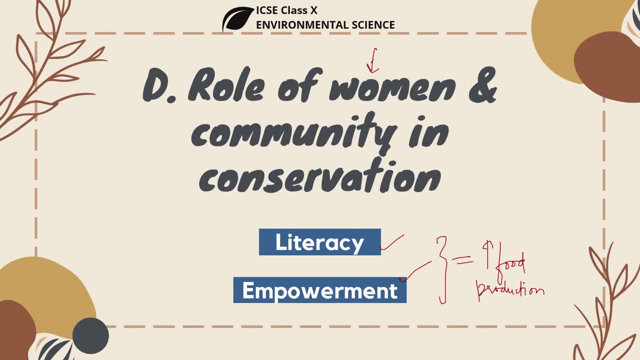 take part in jobs like they go for daily wage laborers, or they may be involved in trading, in selling or, you know, say producing the vegetables, the fruits and other compounds. or they may even be farmers. we do have women farmers as well, so ensuring that they are literate and empowered will help us to manage the 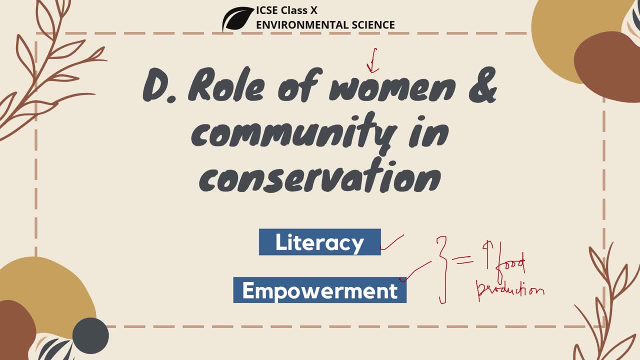 natural resources in a better way. We even have several data where the forest conservation has been, you know, initiated by village women, like, for example, the Chipko movement. women played a major role in it, so they were the ones who ensured that the trees were not cut. 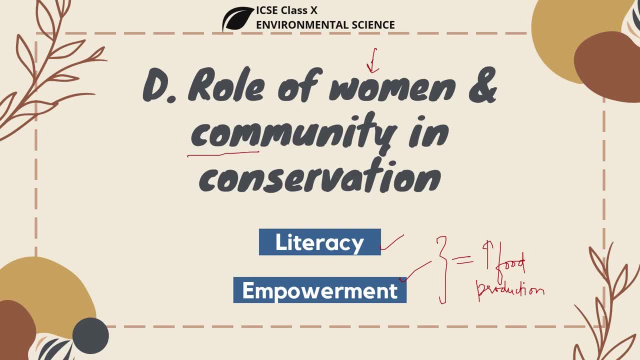 even community, when we see. community-based conservation is also very, very important and it is being utilized in India because community will get actively involved in. in fact, some control is given to the members of the local communities and they are the ones who help in conservation of a particular forest. 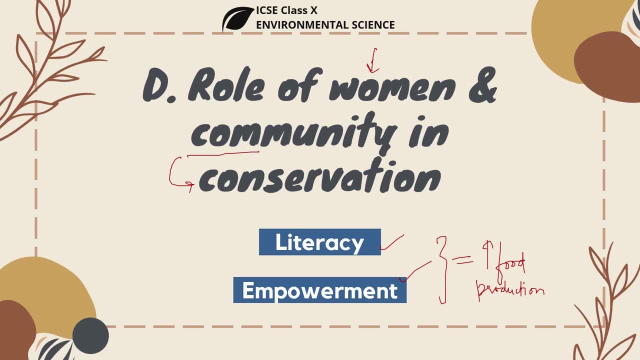 or a particular land, for example, nature worship or having sacred groves is an example where people do not cut down the trees in a particular region because they worship that, those trees or they consider that that area to be very sacred. so even that is an example by which we can use. we can. 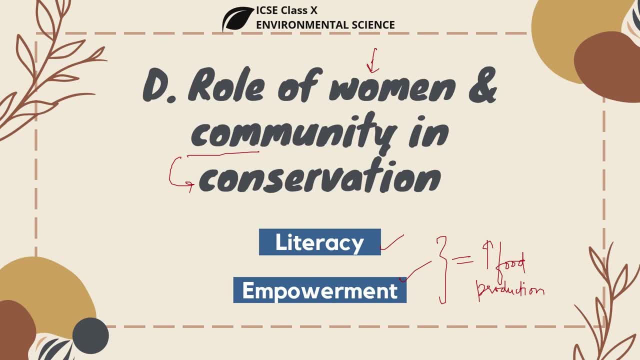 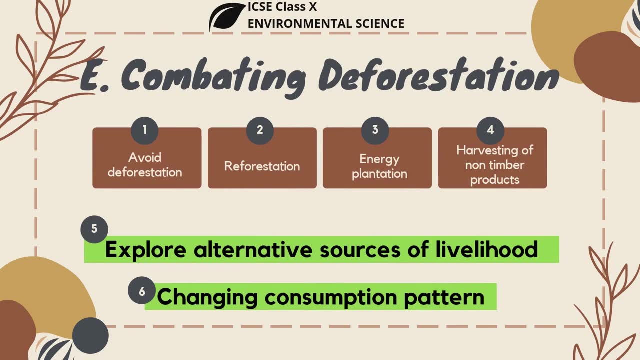 involve the community in conserving a particular region. The next we have in your syllabus is combating, or combating deforestation. now, deforestation is where we have, you know, incessantly cutting down trees, destruction of an indigenous forest or a woodland for economic value. so you use those trees for converting that land. 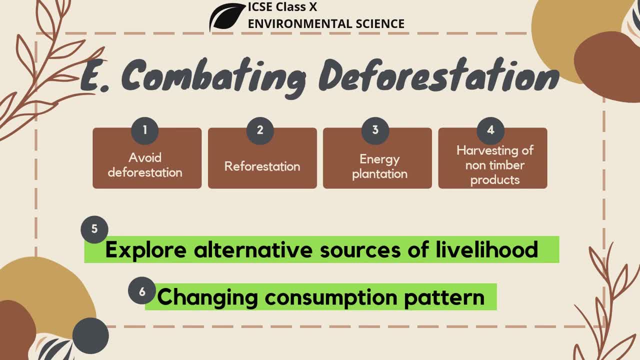 into some other purpose or you use those that timber itself is being used for some particular economic value. The main causes of deforestation are is because of urbanization, it is because of mining, it is because of, you know, having expanded infrastructure. we want to build dams, we want to build roads. that, again, is a 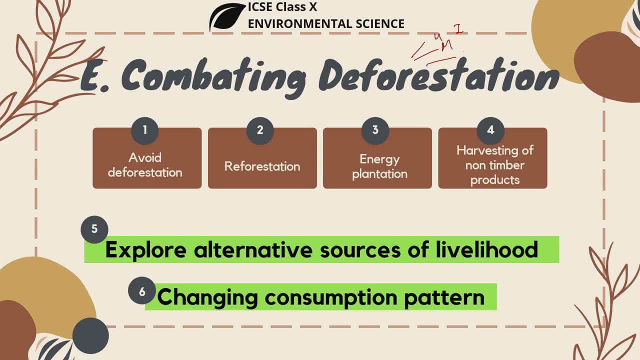 cause for deforestation. Deforestation is a major cause for deforestation. Agricultural expansion: we need more food for growing more crops. we need more area. so expansion of agriculture, raw materials for industries- all of these are the reasons why forests are being cut down across the world. it's not just 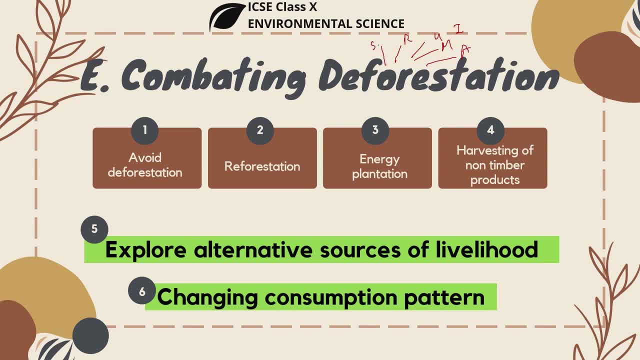 India, everywhere, even shifting agriculture, which is a practice where some communities cut down trees, then they grow some crops over there. they leave that area, go to another area, cut down the trees over there. that's called a shifting agriculture. it is seen in some of the states in India as well. so 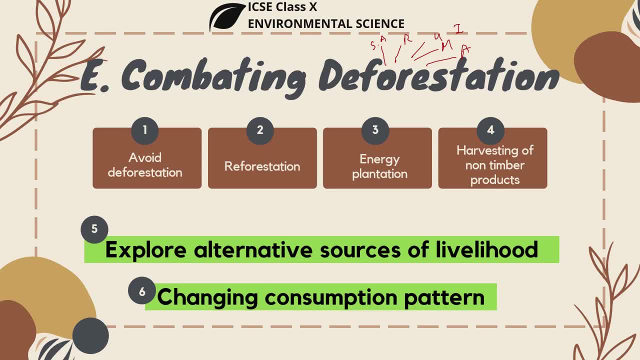 these are some of the reasons why deforestation is happening. These are some reasons why deforestation is so rampant and we need to control it, because if there are no trees, we know that it can cause, you know, a range of environmental effects. it can cause a cascade of effects, for which will ultimately harm humans and even the biodiversity. 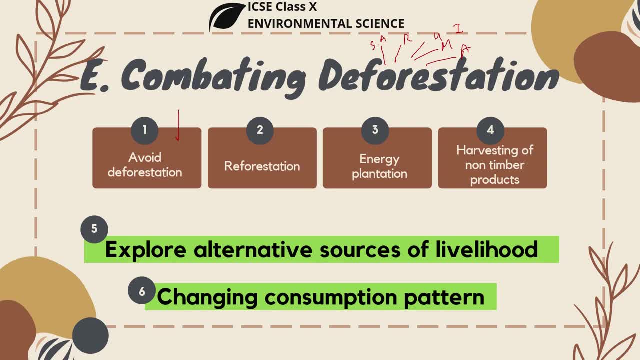 So the first, easiest way is to stop the deforestation. we have to avoid it, we have to, you know, look for alternatives and we need to stop cutting trees first. Secondly, we need to stop deforestation. We need to start planting trees. so reforestation, restoring, regenerating, 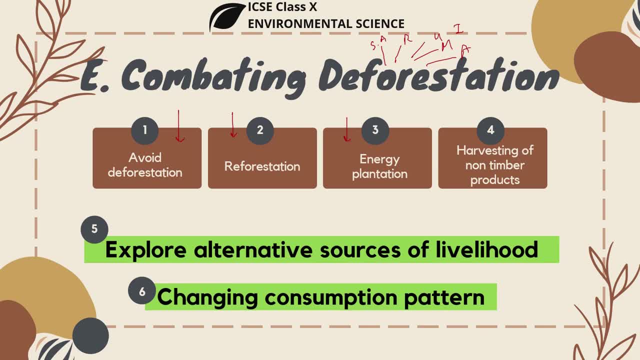 forest is important. energy plantation is the next part, where you grow species of trees or shrubs that can be harvested in a short time and it which can be used as firewood or you know, which can be converted into fuel like ethanol. so they are, there's a dual role over there. you are growing trees which can be harvested. 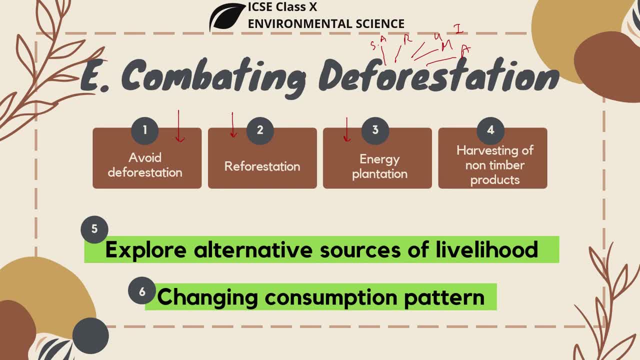 quickly and they are usually, you know, going to protect. when there are trees growing over there, they are going to protect the lands from erosion as well from floods and floods. It also generates rural employment. so energy plantation is very useful because you get the trees, they grow quickly, you can use them for whatever need you need you want. secondly, they 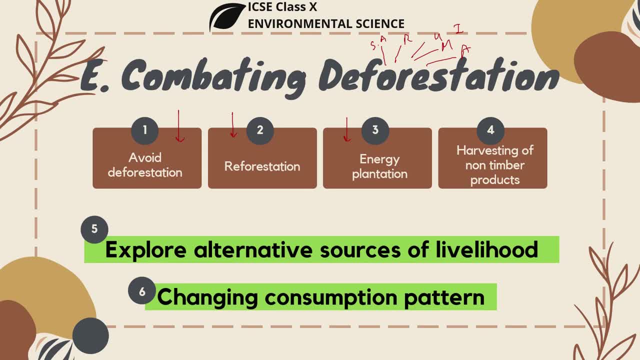 protect from erosion. and third, they generate employment. so energy plantation is something that is being looked into actively. The fourth one is to harvest the forest for non-timber products. so instead of using the forest for wood, avoiding the wood usage, instead of wood you use the forest for. 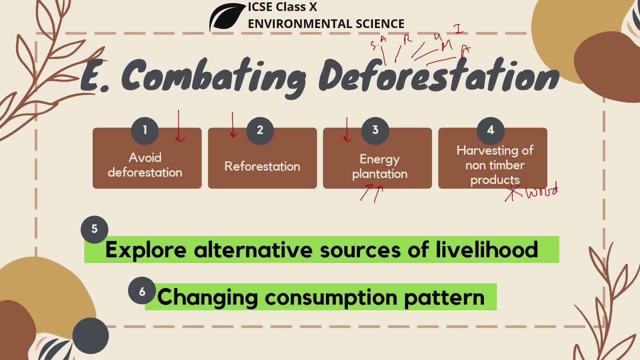 other products like nuts. So instead of using the forest for wood, you use the forest for other products like nuts or seeds or mushrooms or berries or- you know the foliage- for medicinal plants. so instead of cutting down the big trees and using the timber, you use other. 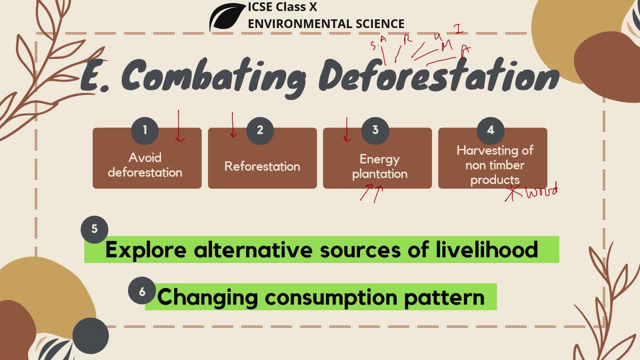 products from the forest. that will also improve the rural economy, the markets. it will keep the traditional knowledge alive as well, so this also helps us in combating the deforestation. The next part: these two what have been written are the very important ones, so we need to explore alternatives. you know we have. 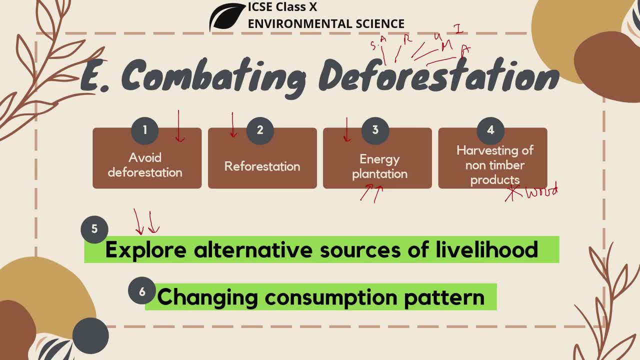 to look for alternative sources of livelihood. there are many tribes, tribal people, who derive their basic requirements like food, fodder, fuel, from the forest. we need to provide them with an alternative livelihood. you can't suddenly go to the tribals and tell them: stop cutting forests because you have done enough damage to the forest. you cannot tell them not to. 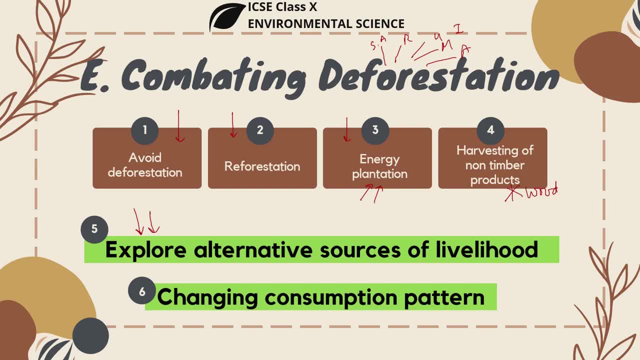 use. you need to provide them an alternative source. only then can we stop cutting down the forest. We have to teach them skills like masonry or carpentry or pottery- handicrafts- anything that will help them to sustain themselves. these have to be taught to them. 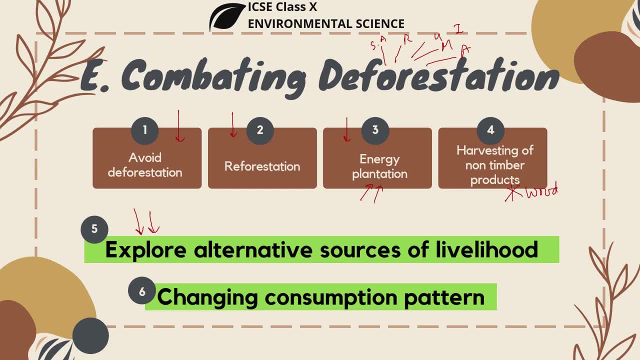 that they have lesser economic dependence on the forest. they are also being you know you. they don't overuse the forest or degrade the forest. you need to provide them with alternative sources of livelihood. there has to be a change in the consumption pattern. this is happening, but 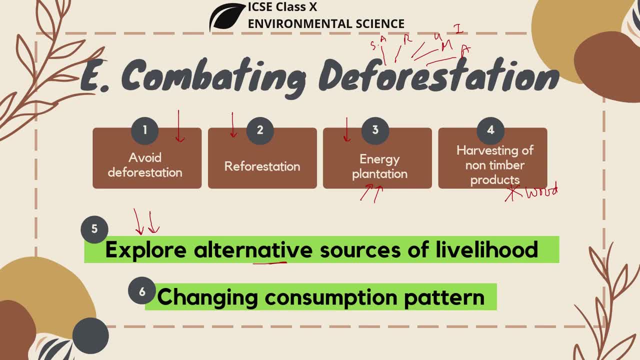 happening at a slow rate, but we need to continue doing it. how? what does that mean? you consume less. that's the easiest way, so you cut down the greenhouse gas emissions because you're consuming less of the timber you are. you don't need to cut down forests, for one of the examples could be: 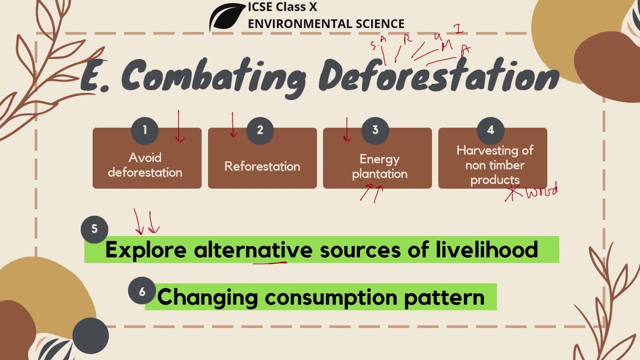 recycling the paper. so we'll look at that in detail in the next slide. so you recycle the paper, you balance the wood that is taken out. so if you're cutting a number of trees, you ensure that new trees are also being, you know, planted immediately. you buy used wood products, reuse. 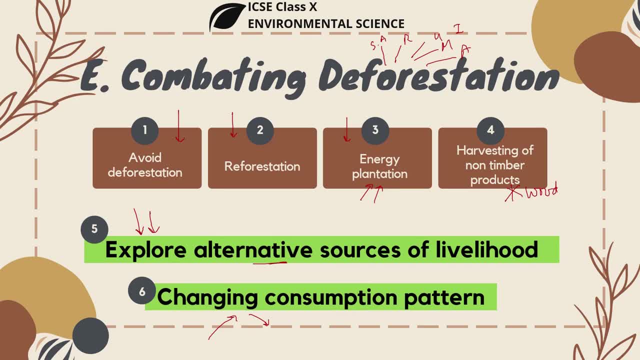 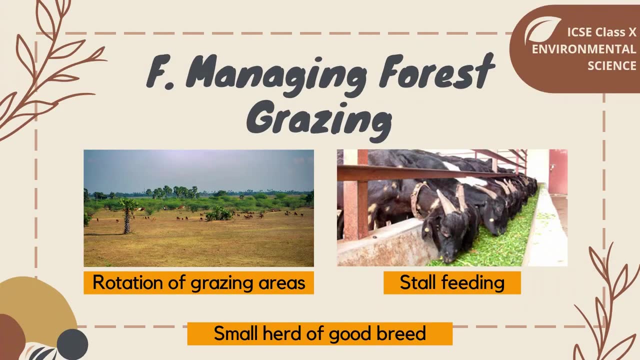 the wood. recycle the wood. recycle the wood in furniture and flooring and you buy less wood. so consuming pattern needs to be changed. only then can we actually bring about some- you know, effect of degrade deforestation, reduce the effect of deforestation. the sixth topic that we have your syllabus is: 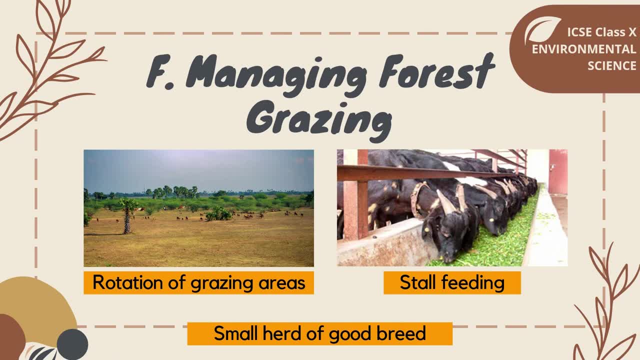 managing forest grazing now, over grazing is a problem. that is, you know, severe grazing that happens for extended periods of time, and this is happening because there's not enough recovery period. you don't allow the plants, the grasses, to grow before that grazing is happening, and this is when the number of livestock is exceeding the carrying capacity of that land or the same. 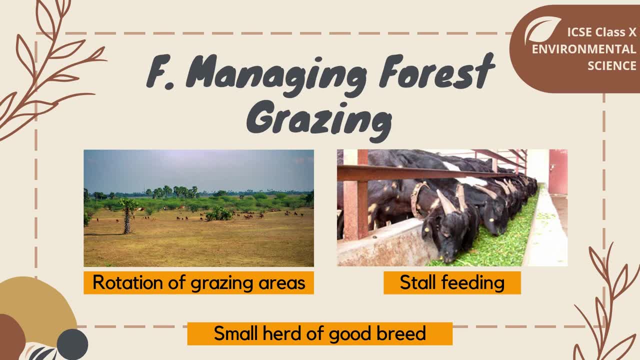 patch of land is being used for grazing. the cattle owners are too poor to grow the land. they're not able to that, are too poor to stall feed the cattle. you know they are not able to provide the food to the cattle in this way. these are all the causes of over grazing, and overgrazing is very, very. 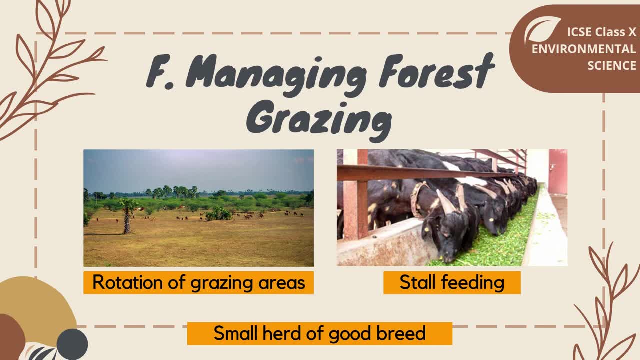 dangerous because it reduces the productivity of a land and eventually it causes the land to get converted into a desert, which is called as desertification. so we need to stop forest grazing, and that has been specifically listed out even in our national forest policy. the control of overgrazing can be done by rotating the grazing areas, choosing different grazing areas, which is to rotate and to overgrazing, which is to control the overgrazing areas, are going to be done by rotating the grazing areas, choosing different grazing areas. Citizen's land registrations, overgrazing are required that the forest is going to get the land and that is made available to the 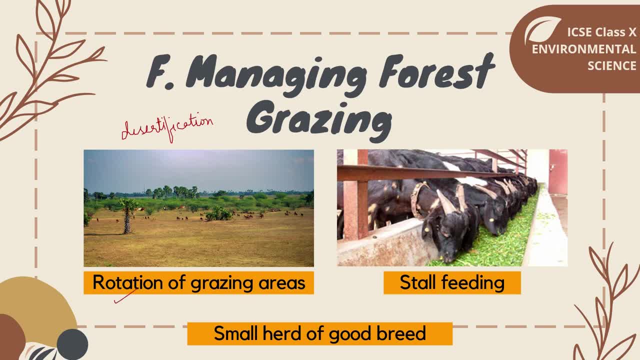 area so that you give enough time for the grasses to grow, encouraging stall feeding in areas where their livestock you know volume is very high, and ensuring that you raise a small herd of good breed so that you know you don't have too many animals over there and you have a small bunch. 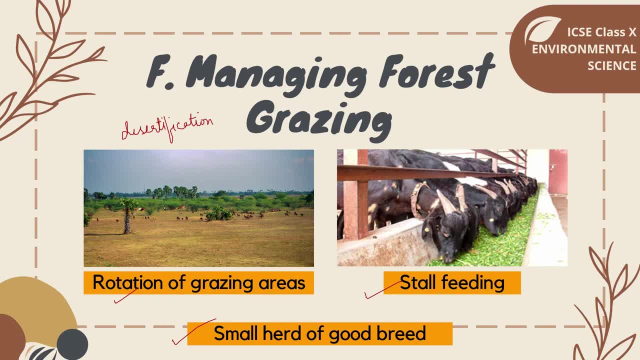 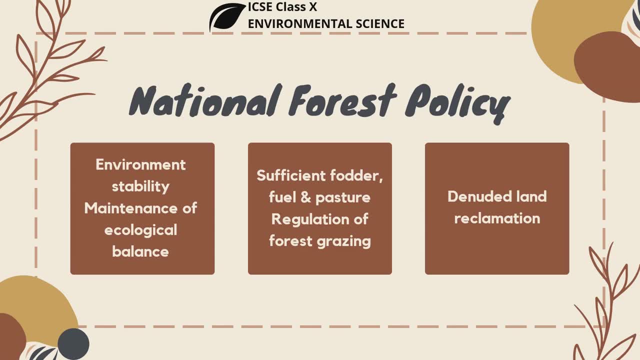 of good breed that is going to give you whatever economic value you need. in our national forest policy policy which was given in 1988, there they have a specific, you know, clause which talks about providing sufficient fodder, fuel and pasture. why? because you need to regulate the grazing in forest. 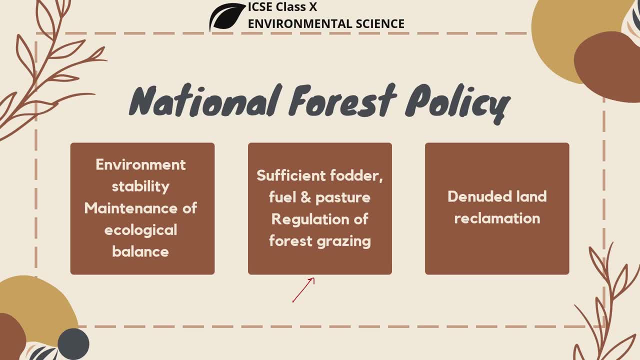 areas, and you have to involve the community for this, so ensuring that individuals or institutions you know they get motivated to undertake tree farming or fodder plants or grasses in the degraded land or the denuded land. that is also one of the ways that the forest policy has told. 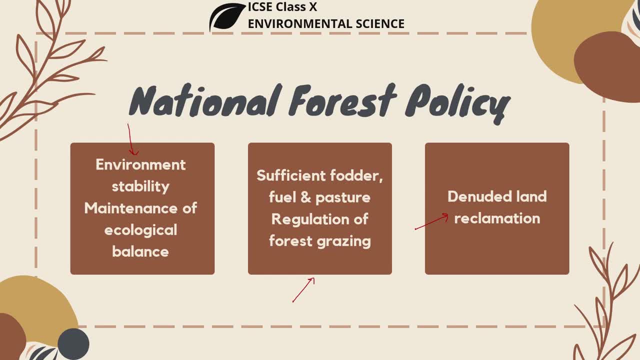 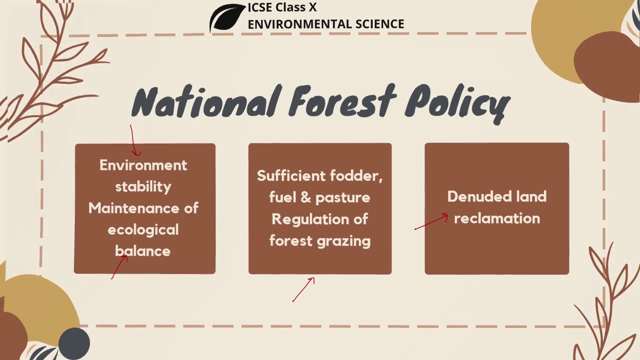 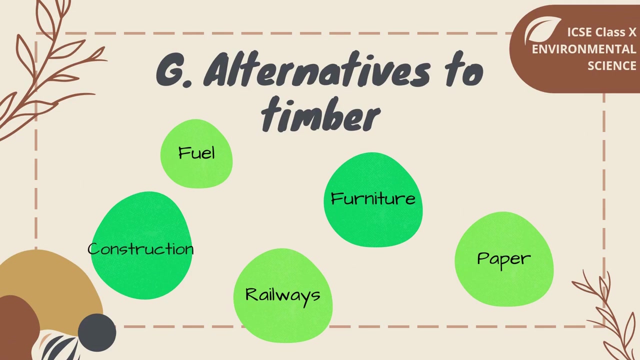 basically, basically ensuring that there is stability of the environment and we are able to maintain the ecological balance. These are the different aims that have been listed out with respect to grazing, with respect to control of forest grazing in the national forest policy. The last part we have is to look for alternatives to timber. So we use timber in fuel in construction. 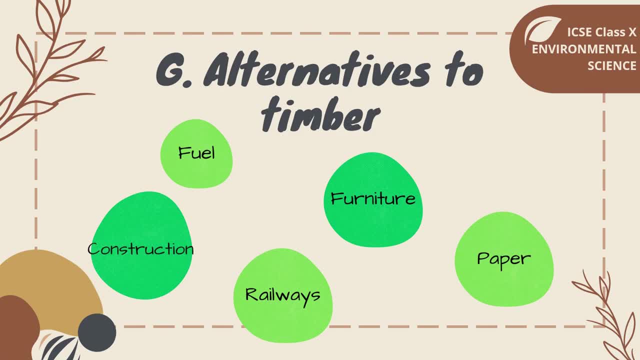 and all of these arenas. we need to look for alternatives. For example, instead of timber in case of fuel, we could go for using dumb cakes, cow dung cakes, dried wood, or look for solar cookers. or we use pellets from sawdust or waste of the saw milling, or rice husk or the oil cakes. 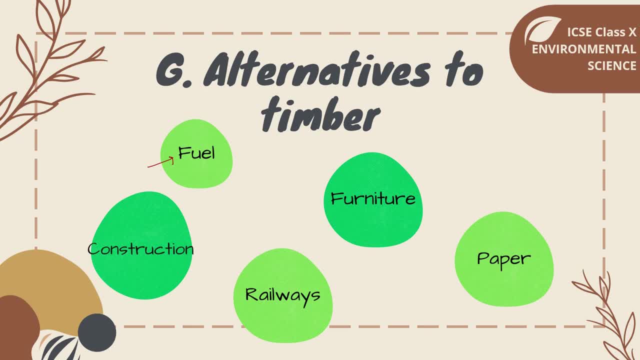 or in some cases, we can even go for kerosene, but then again it's a fuel which has other problems. So, or even we could go for biogas. One way or the other, we need to look for, we need to provide alternatives for timber being used as a fuel. These are some of the alternatives that I have. 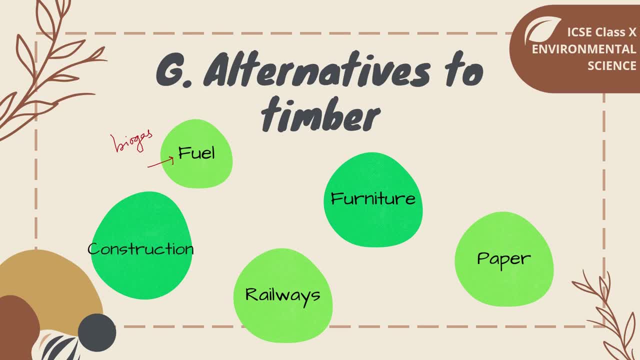 listed out. Timber is also used in construction material, especially in the coal countries, So we need to go for other alternatives like concrete or metal units which have thermal treatment, or the door and window panels need to be used of metal, So we need to look for alternatives to the. 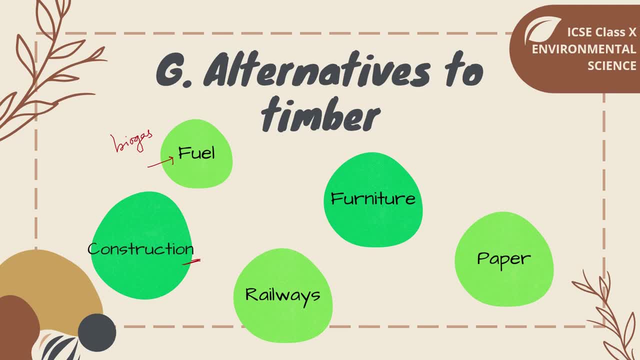 timber in construction as well. In railways, wooden sleepers are used, and instead of wooden sleepers we need, we can maybe shift to concrete or even metal In furniture. furniture is a place where we are using a lot of wood. Instead of that, we should shift to iron furniture or steel furniture. We could even go. 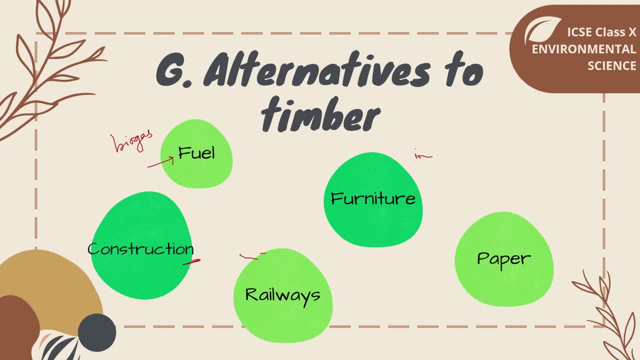 for plastic furniture, So we need to go for furniture which nowadays we even have, you know, furniture that is made of recycled material. Waste material is then recycled and then we are using it as furniture. So we have to look for alternatives to timber, even in furniture. Lastly, instead of 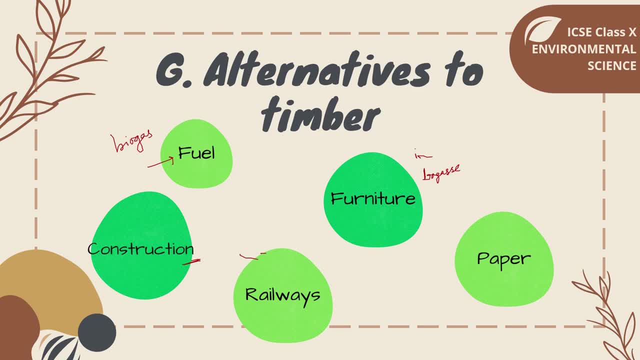 paper. we can, you know, recycle the paper or make paper made of reeds. Instead of cutting down trees, look for the reeds or bagasse, or, you know, you recycle the paper. You can even do it four to five times. Use scrap paper, Use to make cardboard or packaging industry. So there are different.